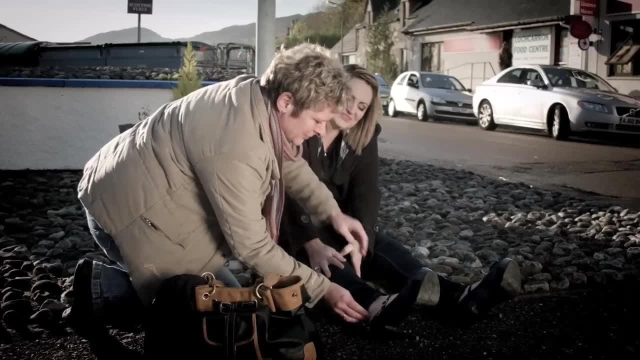 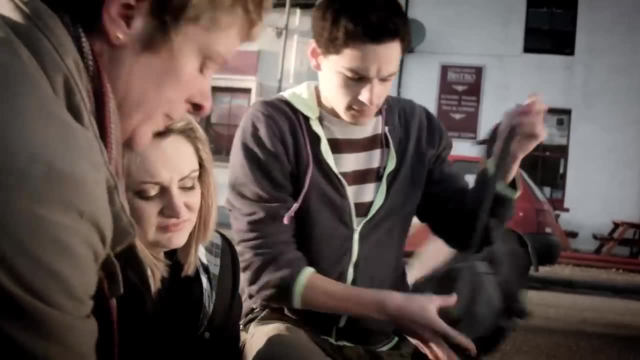 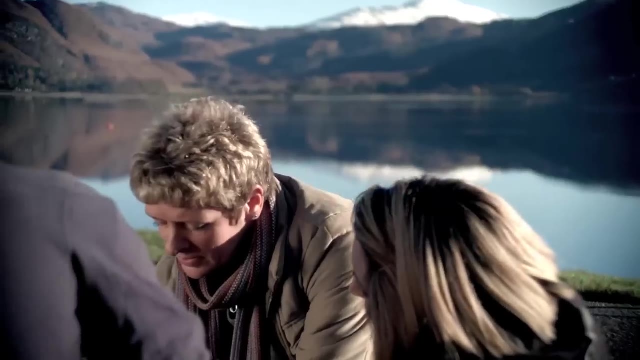 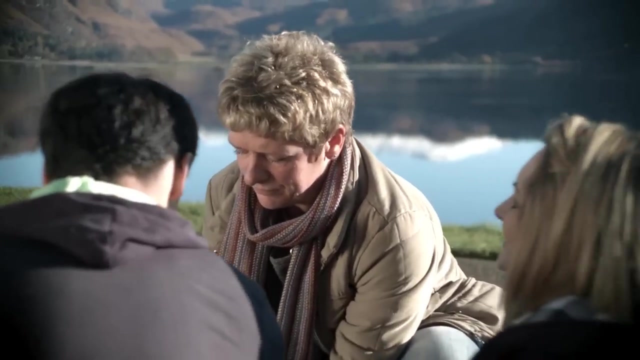 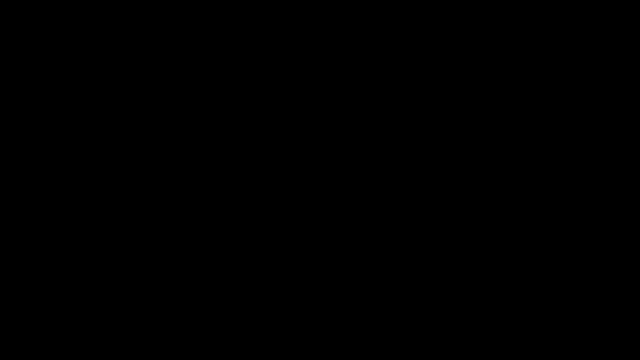 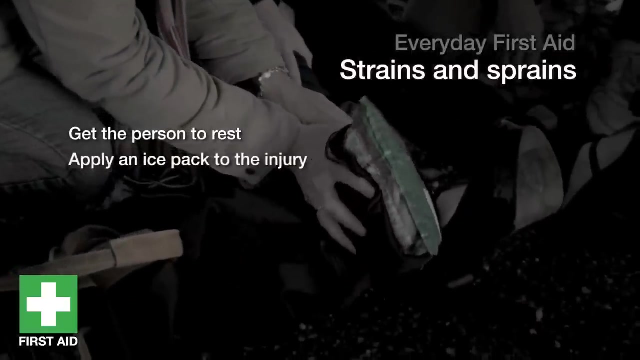 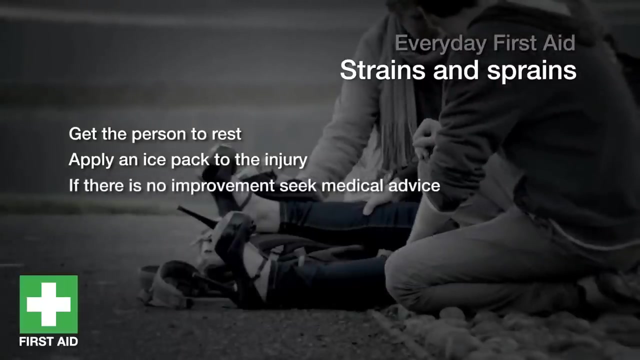 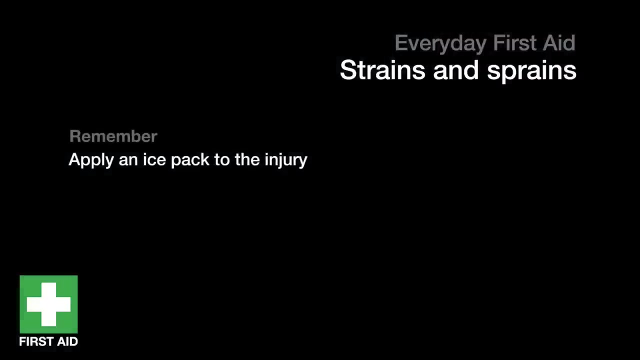 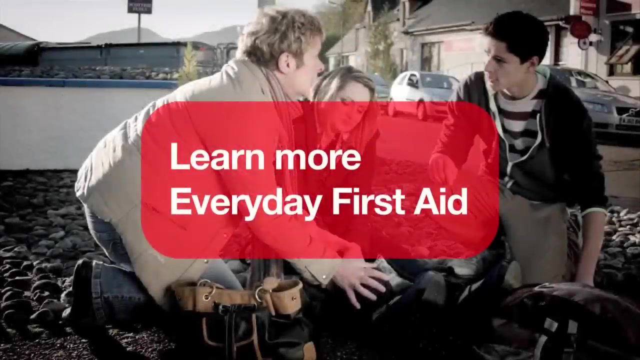 exactly does it hurt? It'll be okay, Thank you. Okay, this'll help to keep the swelling down. Let's get her leg off. Thank you so much. Thank you, Thank you, Thank you.